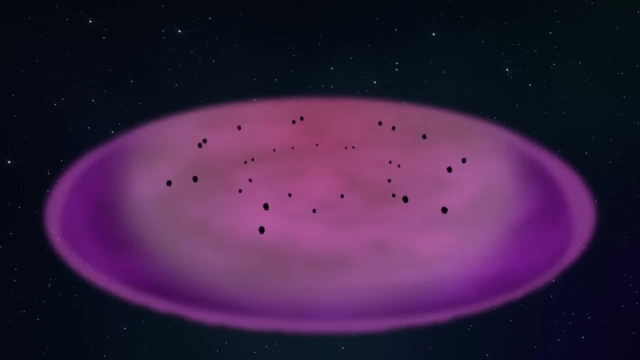 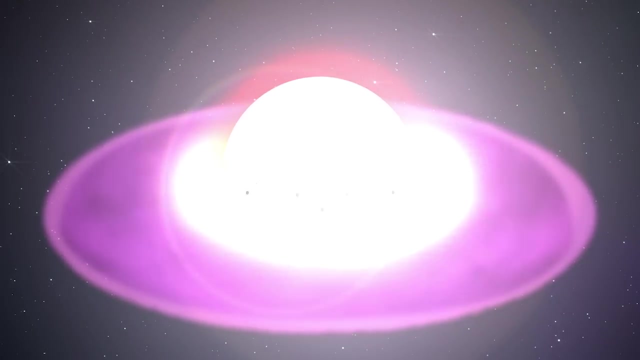 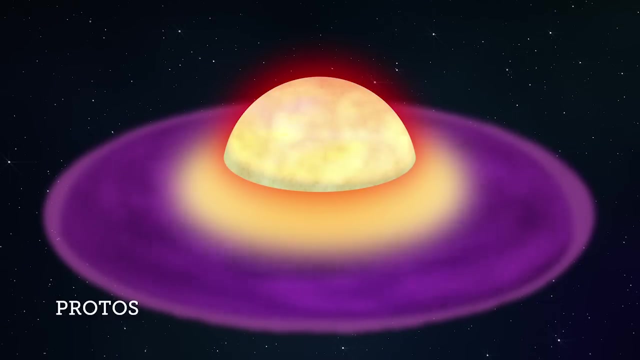 the gravity also increased and, as a result, the temperature continued to rise. A ball of hot gas formed in the center of the accretion disk, creating a protostar also known as the Sun. Finally, when enough gas gathered in the center of the protostar, the pressure generated enough. 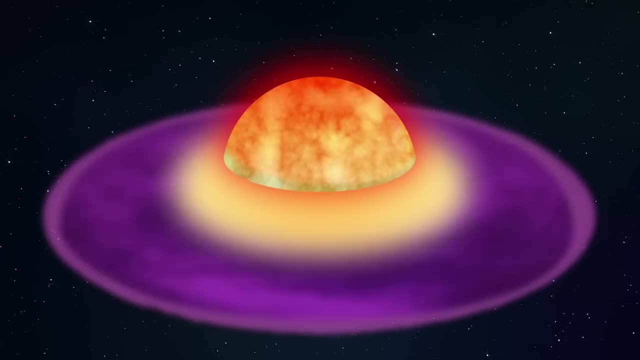 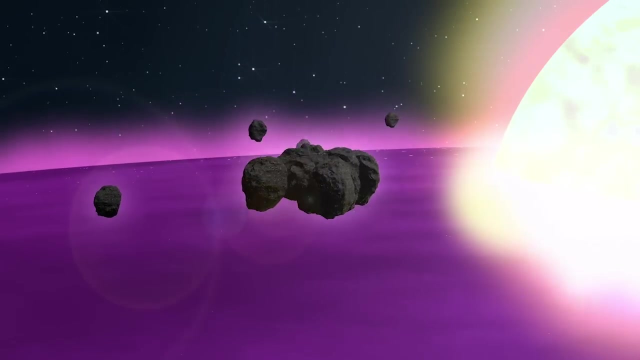 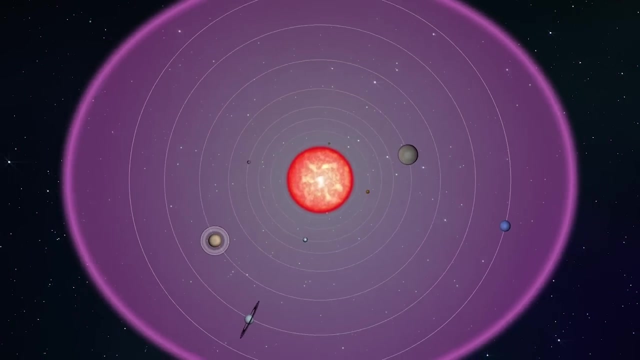 heat to fuse the atoms forming a star. Outside the star, matter was forming into clumps of gas, dust and rock, which created protoplanets. These protoplanets continued to grow as they trapped material in their gravitational fields. Because the protoplanets all formed from the same cloud of gas and dust, they travel. 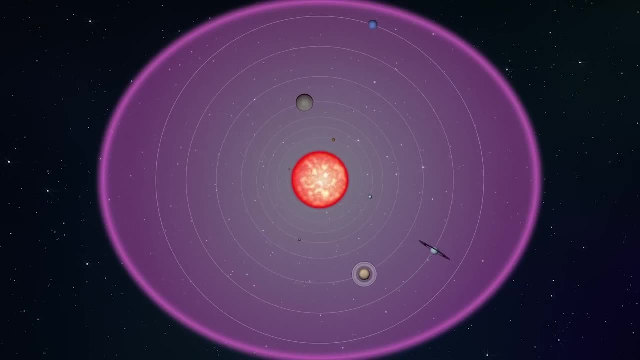 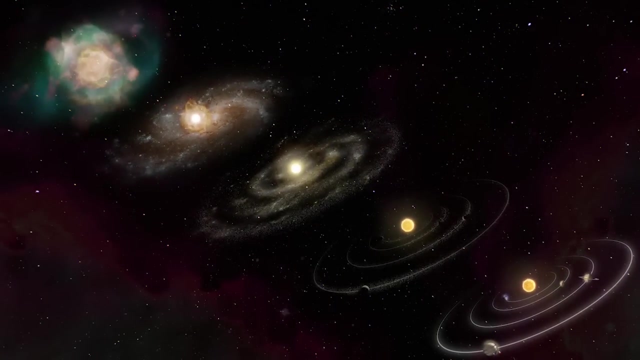 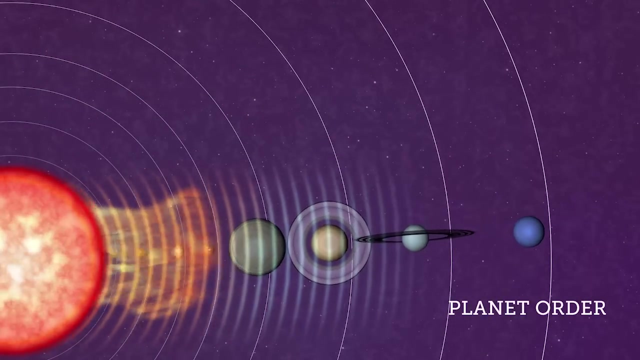 around the Sun in the same direction and in the same plane. The nebular hypothesis also explains how the planets are arranged. The heat and solar winds caused by the Sun swept the lighter gases farther out into the developing solar system. This is why the rocky terrestrial planets—Mercury, Venus, Earth and Jupiter—are. 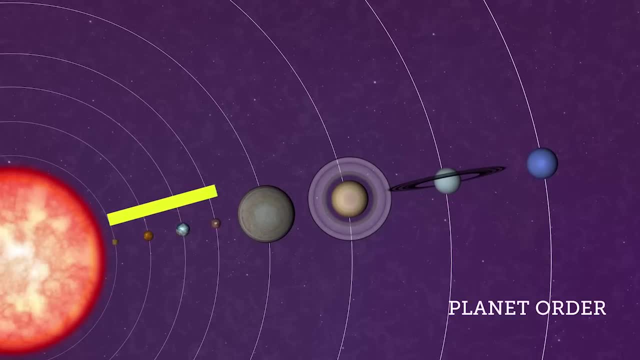 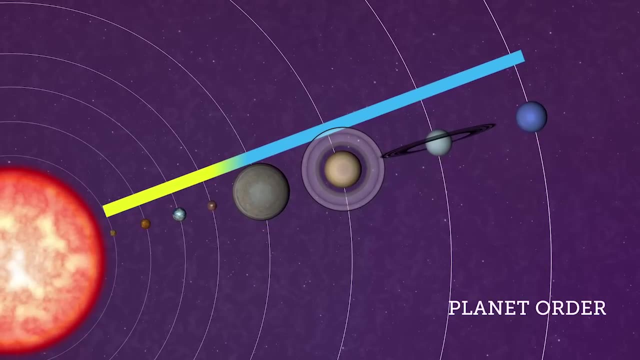 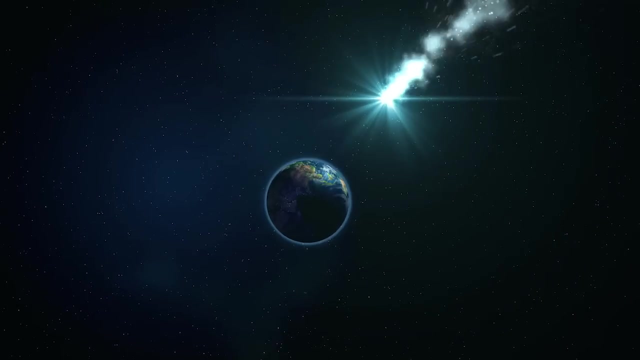 located closer to the Sun. The gas giants—Jupiter, Saturn, Uranus and Neptune—formed in the cooler outer region of the solar system. The solar system continued to evolve even after its initial formation. Large asteroids slammed into planets and the planets themselves differentiated into 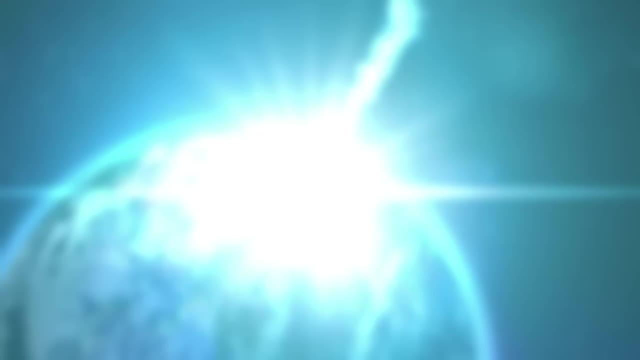 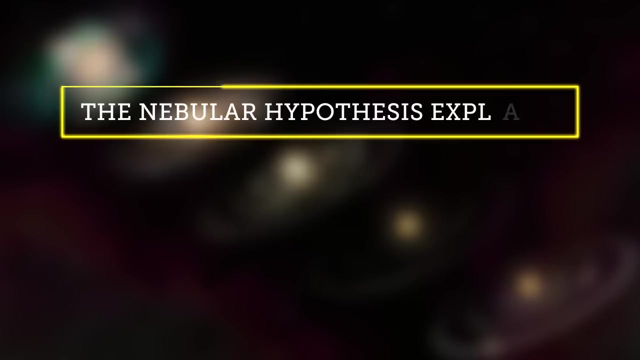 layers as they slowly cooled. Although the nebular hypothesis cannot be derived from the nebular hypothesis, it is directly tested. It is a useful description for how a solar system forms. It explains why planets and the star they orbit usually spin in the same direction and